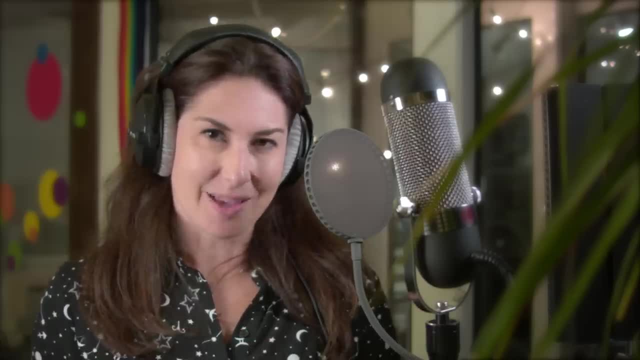 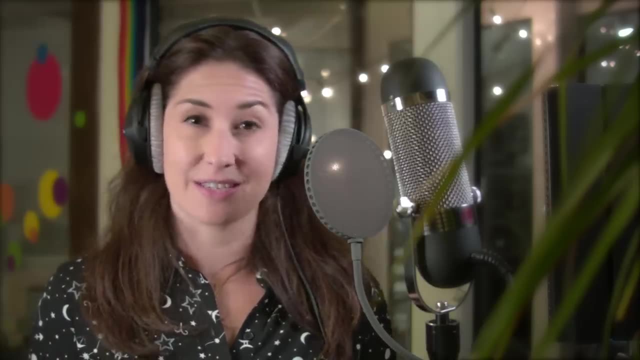 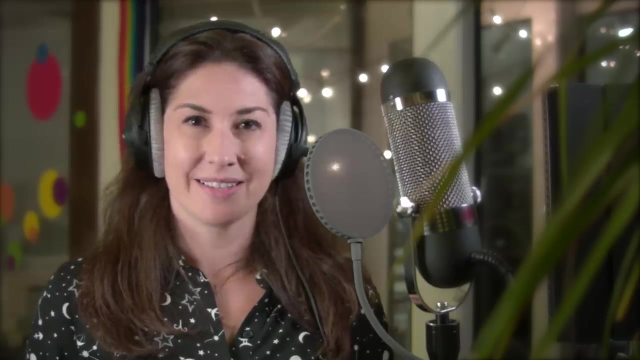 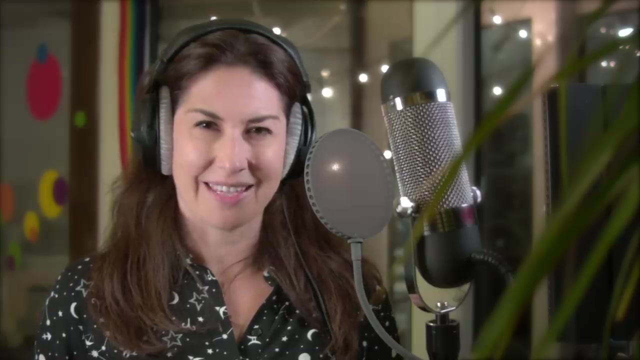 Okay, Now take a moment to do any fidgets or wriggles, just so you feel happy to be still for the next few moments while you enjoy our Peace Out time. Once you're relaxed we'll begin. Let's see if we can notice our breathing. Can you feel it? It goes in through your nose and then out again. 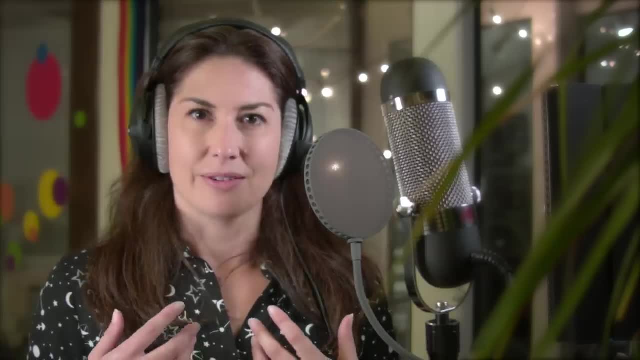 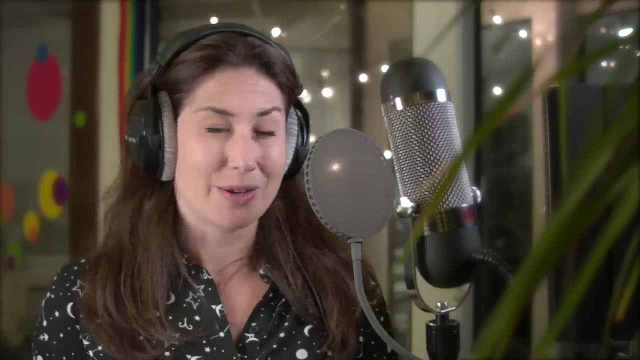 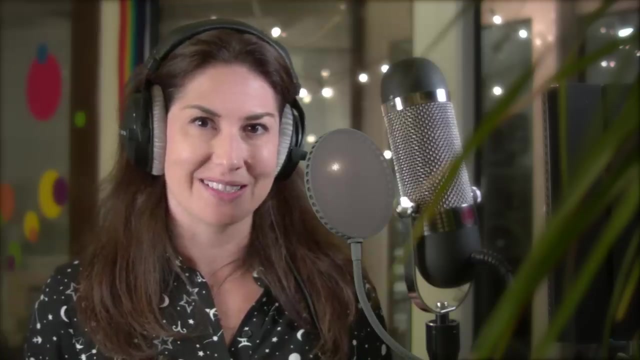 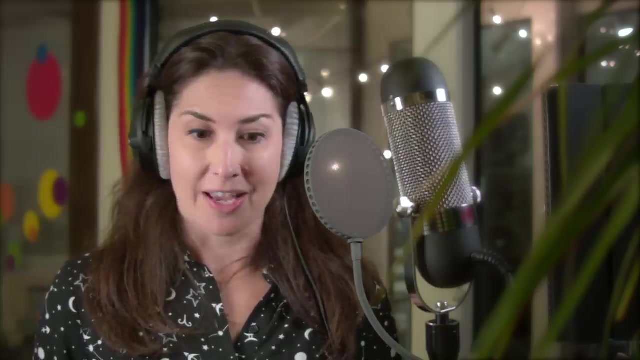 In and out. It might be very quiet and small so you can hardly feel it at all. But see if you can by really concentrating on it. I find it easier when I close my eyes. Give it a try. Let's see if we can breathe in. 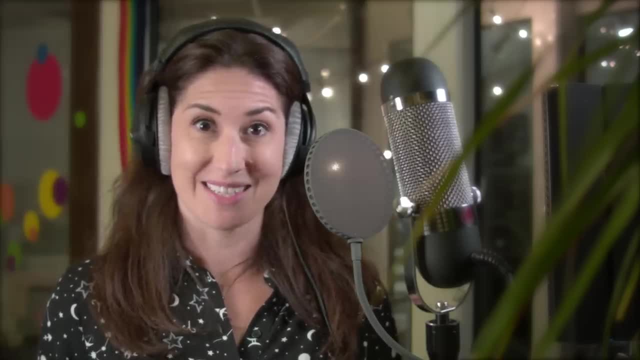 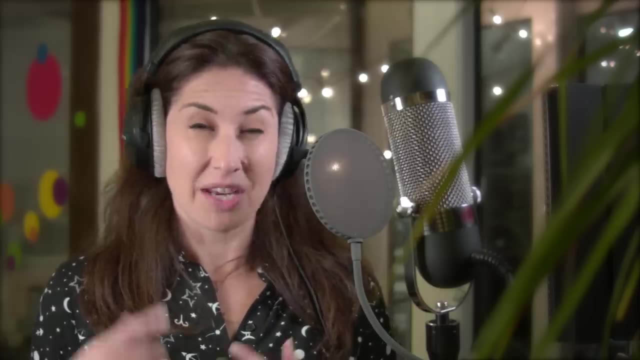 Let's see if we can breathe in and out. Let's see if we can breathe in and out. Let's see if we can breathe in and out out five times, Going slowly. just following the breath, You might notice how your mind 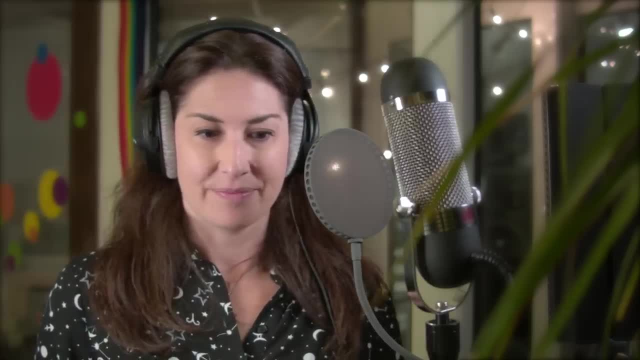 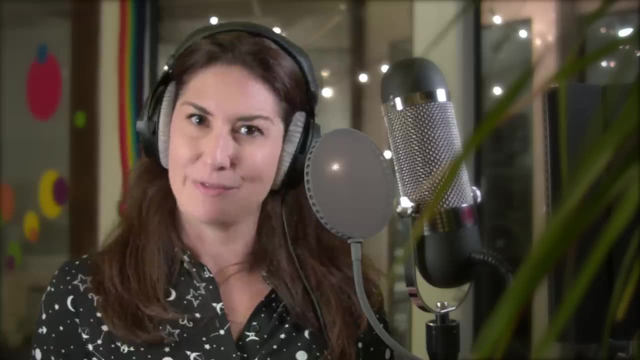 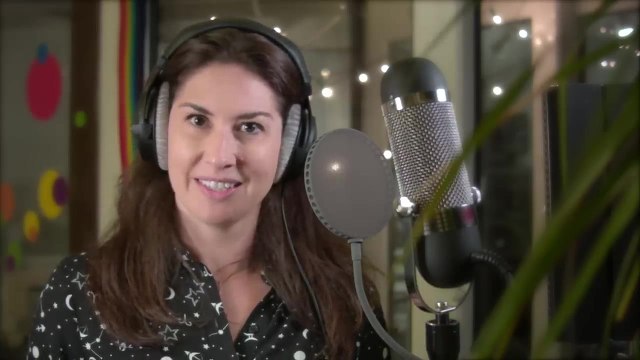 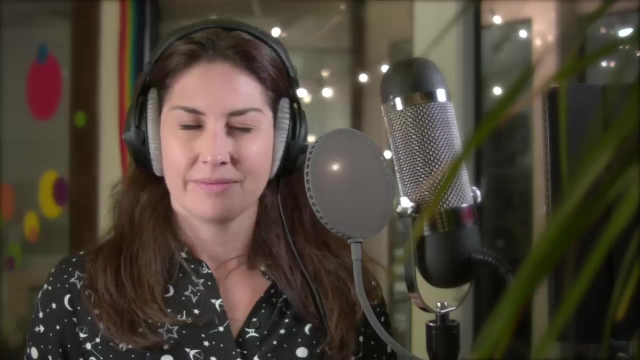 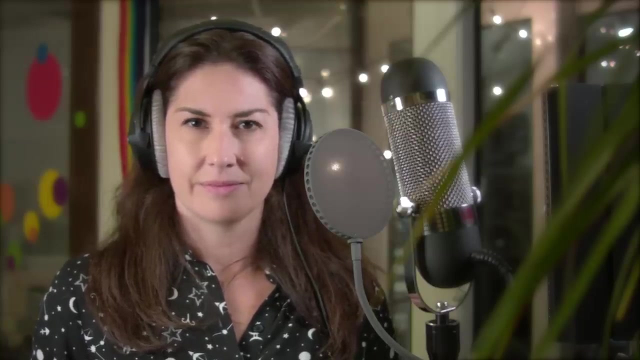 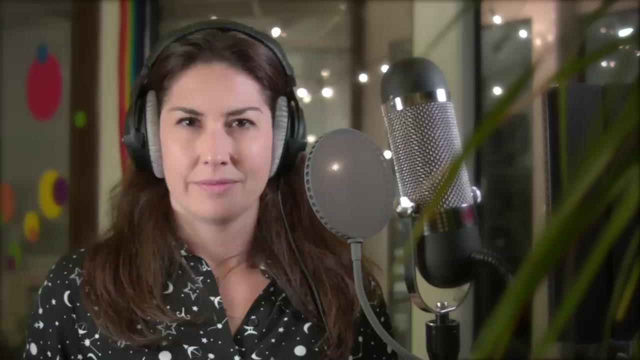 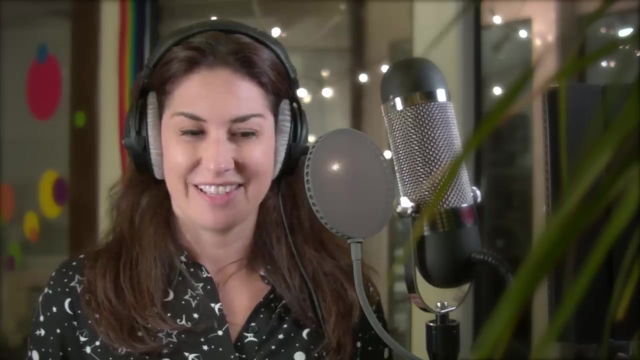 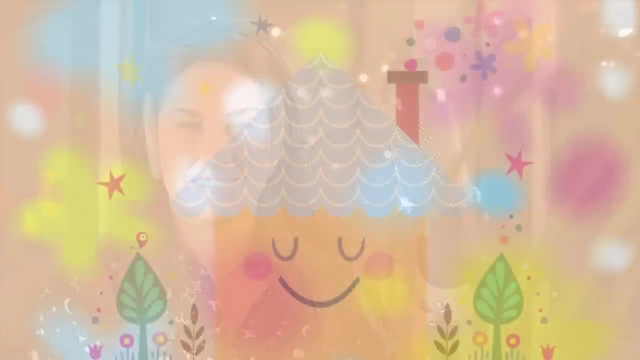 makes you think of other things. If this happens, don't worry, That's what our mind is supposed to do. Just see if you can come back to the breaths in and out five times. I'll do it with you. Well done Now. if you haven't closed your eyes already, slowly close them now. This means your 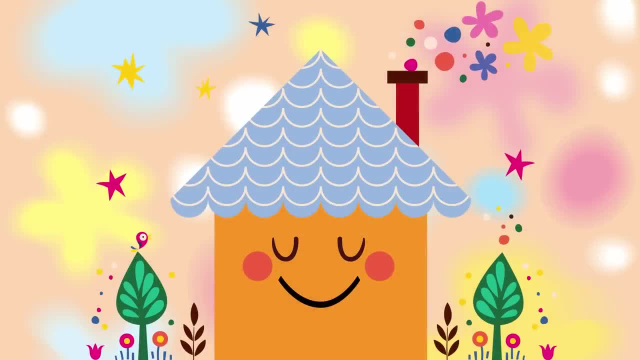 mind can become your movie screen and you can make pictures appear as you listen. Imagine you are walking down a street you know very well, But then you spot a house that you hadn't seen there before. How strange. You go and have a closer. 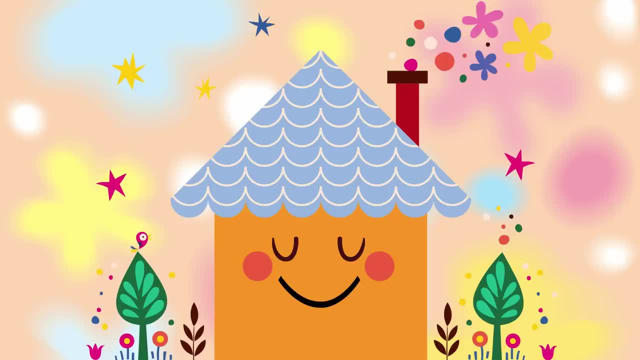 look and notice the door is open. So you take a look inside. The first room you come to has a picture of an eye on it. An eye, This is the room of sight. What you see is a picture of an eye on it. 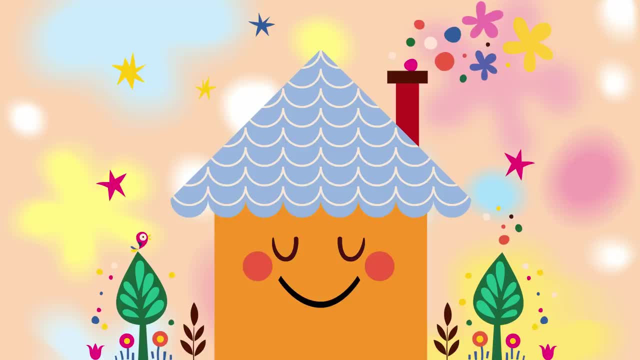 You see your vision. Inside there's all sorts of stuff and old bits and pieces. Imagine all the things you have seen. You can see it needs a good clean. So you get to work filling up bags with all the junk, blowing all the cobwebs away, dusting, sweeping and cleaning the window. That's better. 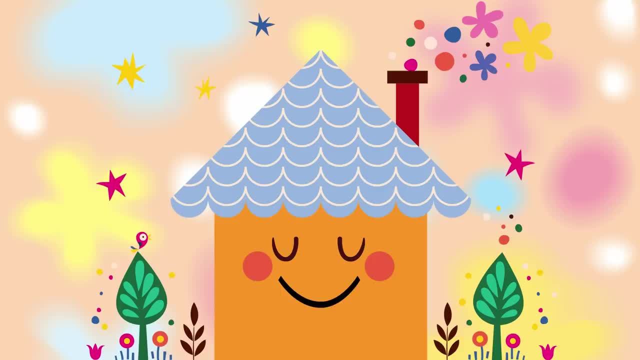 Now you have a lovely clean room And the light is beaming in through the window. You feel good as you leave the room of sight and now come to a door with an ear on it. An ear, The room of hearing – your sounds. 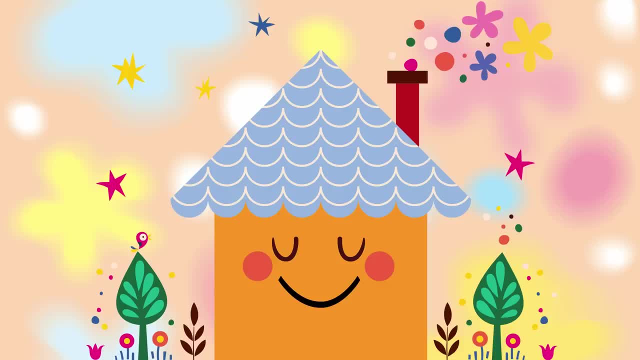 Inside. you find it's noisy, with all sorts of clatters and bangs, screeches and twangs all going on at once. You find it noisy, with all sorts of clatters and bangs, screeches and twangs all going on at once. 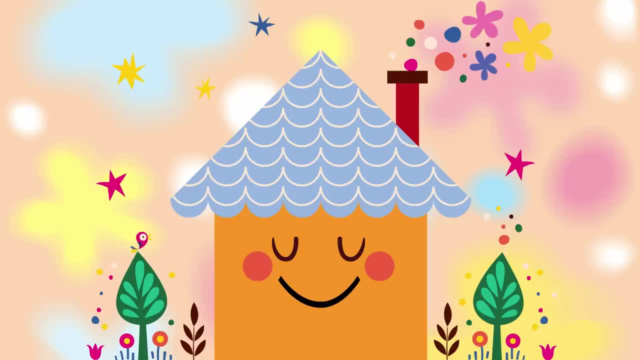 You run to the window and you open it up, an armed car ligger over the Pokémon. You saw something. I don't know what it was, but all those stupid Title 모uloos in the room. You uh see ghosts h ugh, there's some crap up there. 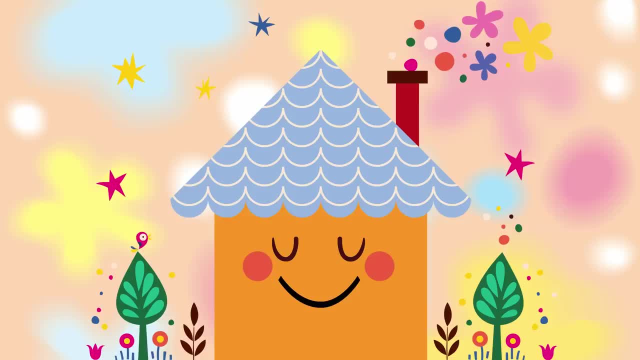 open it up, letting all the noisy sounds out. Now you can only hear your favourite sound or a tune you like. You leave the room of sound and hearing and see the next door has a nose on it. a nose: This is the room of smells. On opening the door, you are met with: 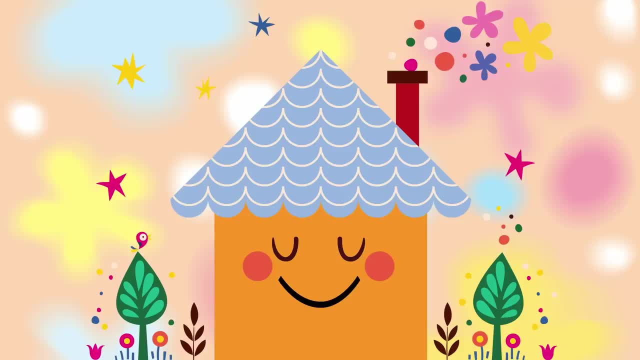 all sorts of smells: food, garbage, fish, clothes, perfumes and animals. You give the room a good scrub and open the window to let out all the bad smells, leaving the space clear for you to smell your favourite smells. You breathe it in and enjoy it. You close that. 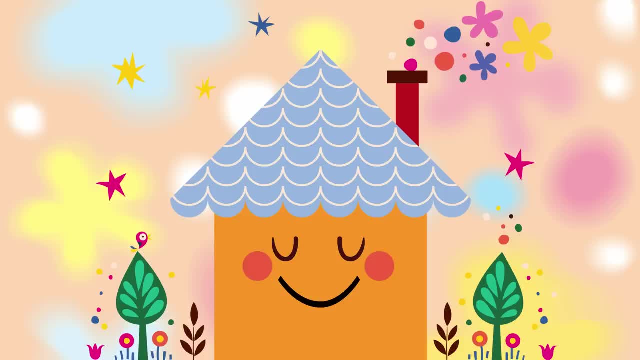 door and come to the next door, next room. The door has a mouth on it. A mouth. This is the room of tastes, But inside is a mush of flavours: Pizza, chocolate cheese, ham, bananas, sausages and ice cream. You. 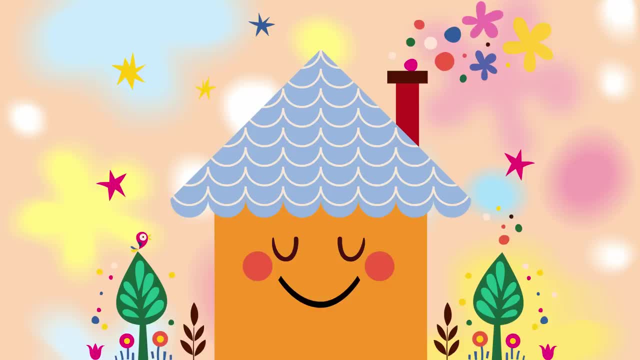 spot a hose in the corner of the room and spray it down, leaving the place completely clear and clean for your favourite taste in your mouth, Mmm. The next room has a hand on it, A hand: The room of touch and different textures. Inside, there's a jumble of textures. 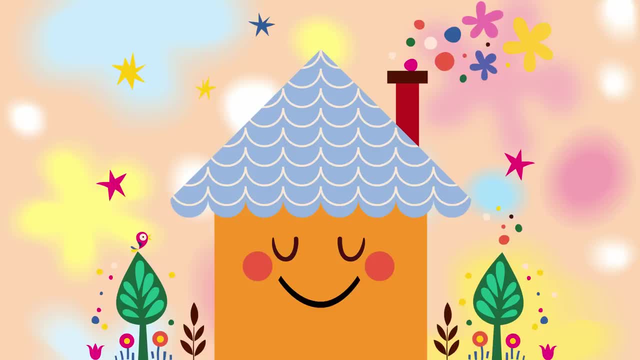 Rough, smooth, wet, furry, soft, spiky, crinkly and silky. You tidy up all the textures and put them all out neatly so you can feel each one separately and enjoy the different feelings you have from touching them. You leave this room and 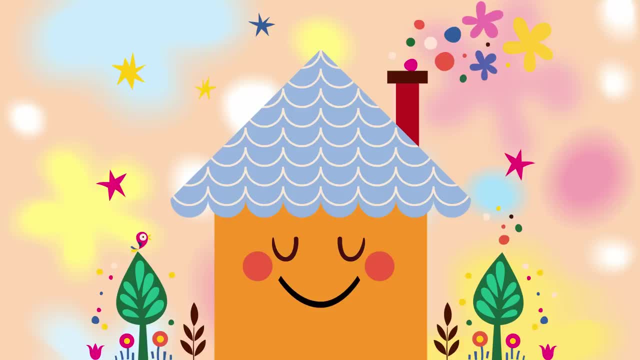 come to a final room which is at the top of the house. It has a question mark on the door. This is the room of your thoughts, Your mind, The place where you dream and have ideas. Inside, you see, it's very messy and untidy. 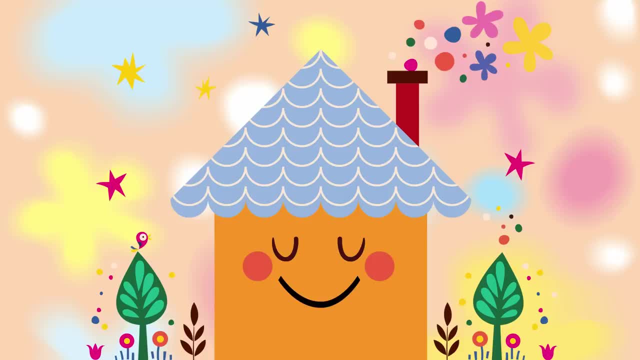 All the toys are out, There are clothes everywhere, The bed is a mess, There's a desk with paper and pens and pencils scattered everywhere. You get the room tidied up, putting everything back where it belongs, Throwing out all the rubbish and cleaning as you go. Now everything. 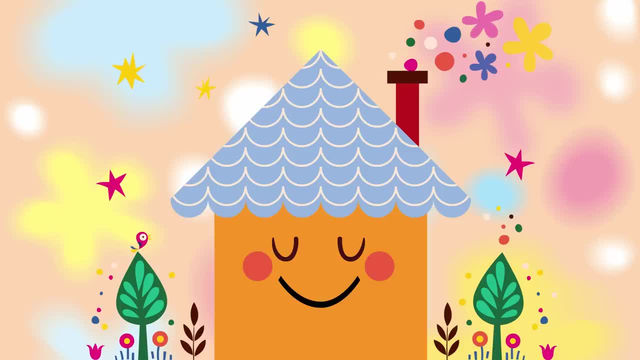 is clean and tidy. You smile and leave feeling clear and fresh. Now your ideas can flow. It's time to go. You walk past each room remembering the different senses, Your favourite sight, sound, smell, taste, texture and idea. Your mind may have sent you off at any time. You leave the house and walk back out onto.